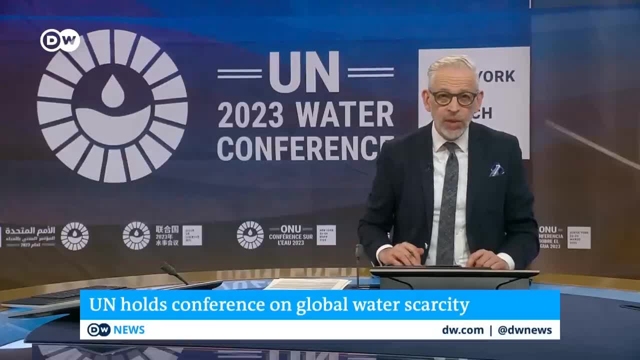 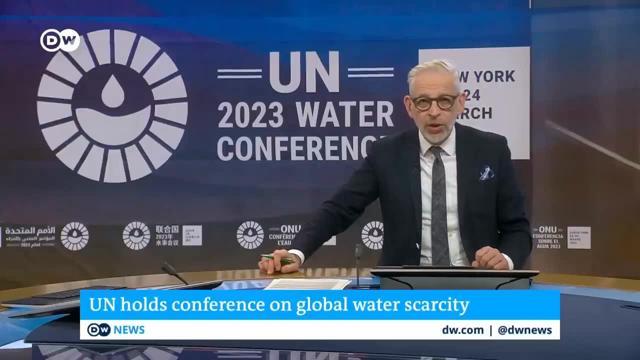 The United Nations is holding a special conference in New York to focus attention on a growing crisis. That's a crisis that's prompted one Australian woman to set herself a unique challenge. 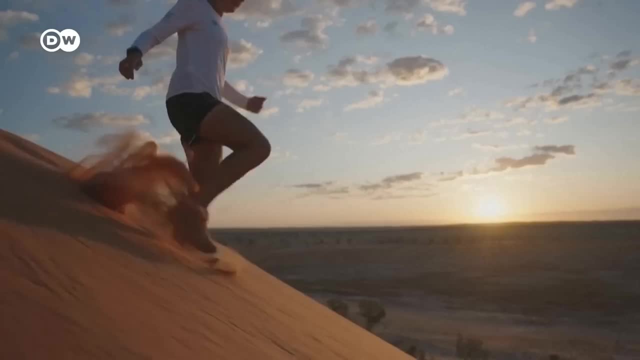 When she noticed that the world was running out of water, Mina Ghouli started running. And she hasn't stopped since. 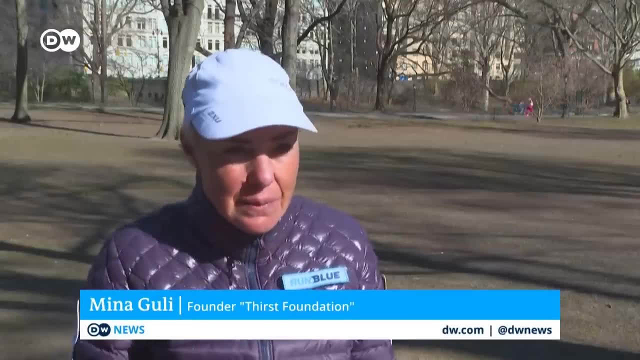 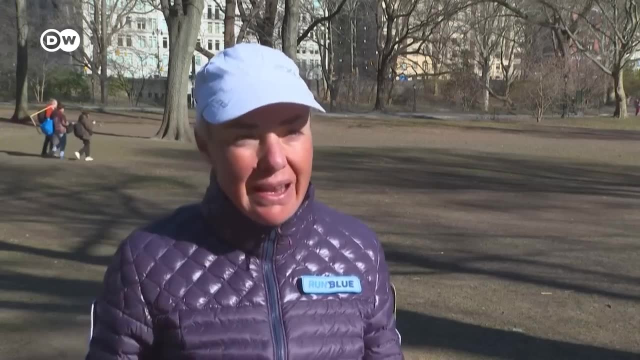 I'm running because I want to take the voices of the people from the front lines of this water crisis and take them into boardrooms, take them into the halls of power and inspire these government officials, these corporate leaders to take action. 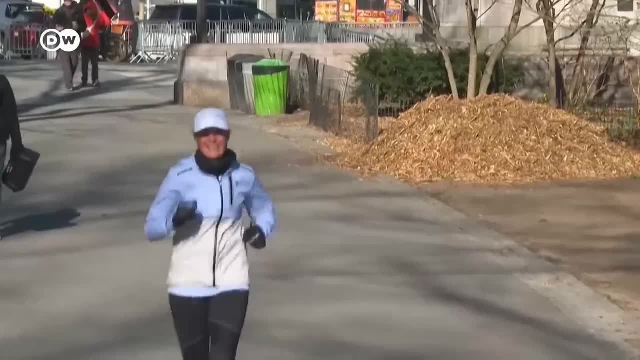 The amateur athlete and activist from Australia completed 200 marathons across 32 countries over the last year. Now she has made her way to New York City. 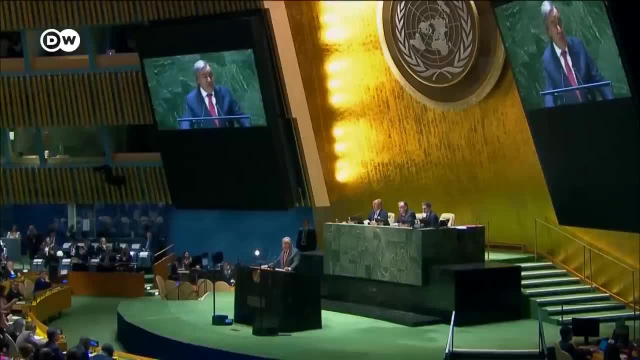 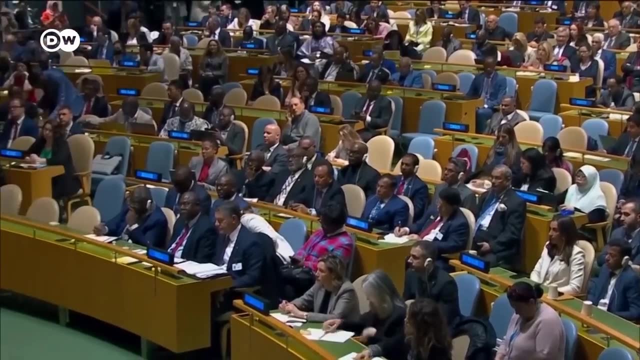 Where delegates have gathered at the UN for a three-day summit to discuss ways out of the water crisis. Around two billion people, a quarter of the world's population, lack access to safe drinking water. 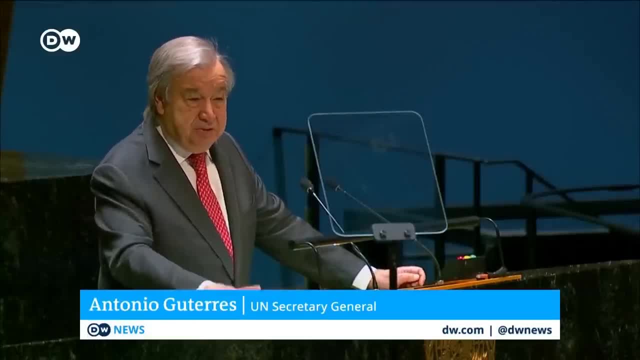 This is more than a conference on water. It is a conference on today's world, seen from the perspective of its most important resource. 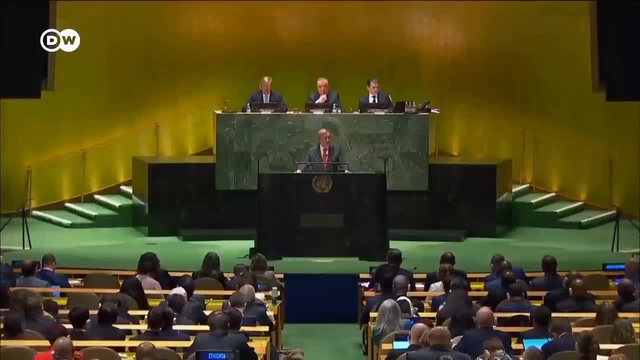 This conference must represent a quantum leap in the capacity of member states and the international community to recognize and act upon the vital importance of water to our world's sustainability and as a tool to foster peace and international cooperation. 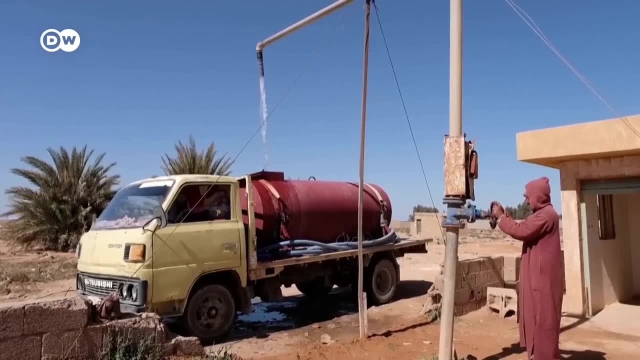 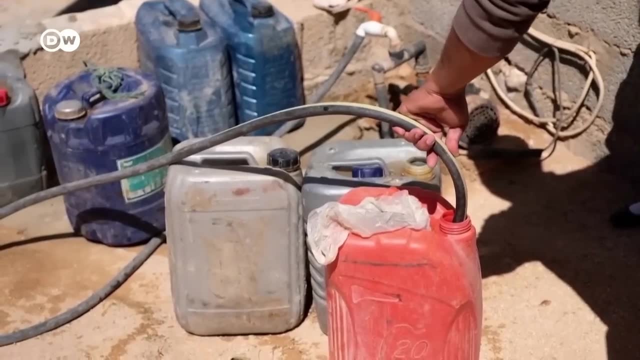 A new UN report shows that the global water shortage is likely to worsen over the coming years, despite the efforts by the international community to make sure everyone has access to clean water. 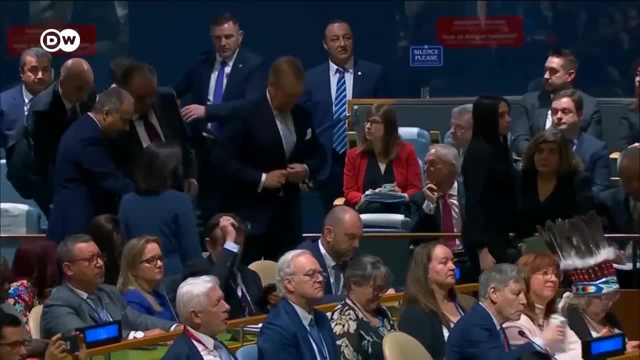 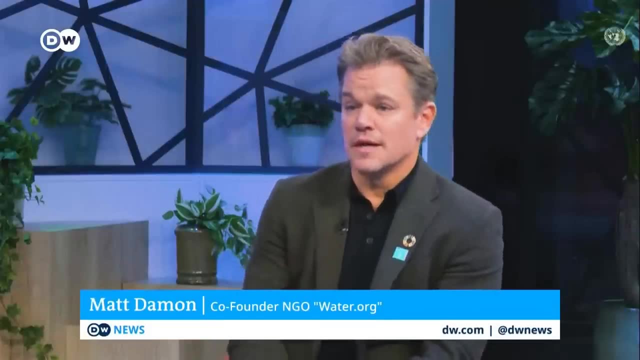 On the sidelines of the summit, some famous faces are highlighting the fact that a lack of water impacts more than just people's health. It touches everything. It really affects women and girls. They are disproportionately affected by this. 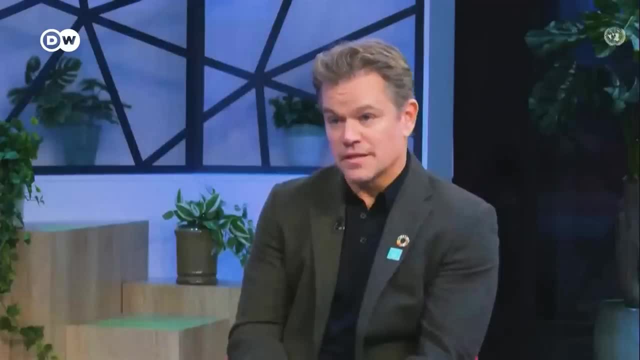 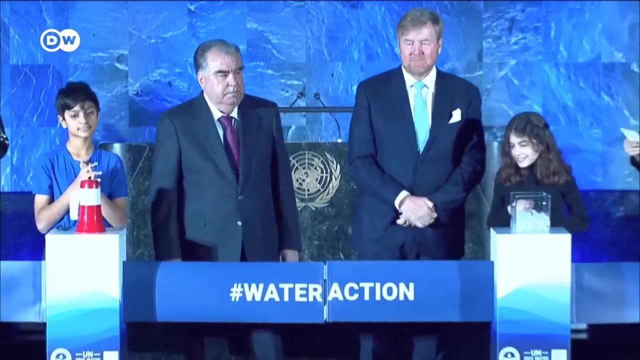 A lot of millions of girls aren't in school because of this, because they're collecting water. The UN wants to guarantee universal access to drinking water by 2030. But scientists warn that the global community would need to triple its efforts to achieve that. 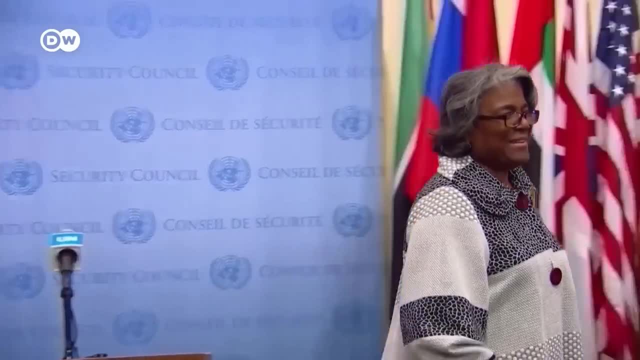 As the summit kicked off, the US government promised 49 billion US dollars of funding to help the global water cause. I think it's easy in places like Paris. Or here in New York City, where we turn on the tap and water comes out. To forget that there is this major systemic global water crisis that exists out there. 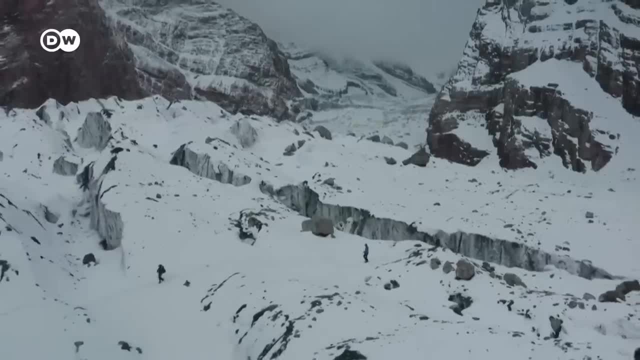 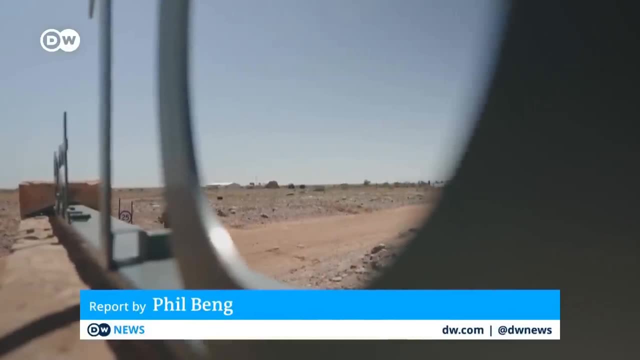 Mina Ghouli has witnessed that crisis herself, seeing melting glaciers and arid regions during her journey. Now she hopes that the world won't turn a blind eye to an issue that in the end will affect everyone, everywhere. 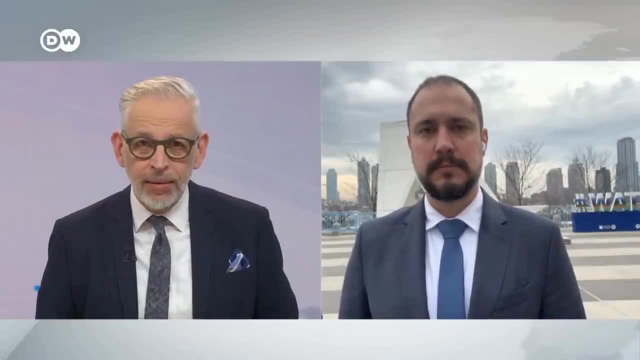 Let's bring in Kaveh Madani. He's a member of the UN. He's the director of the UN University Institute for Water, Environment and Health. And he joins me from the UN Water Conference in New York City. 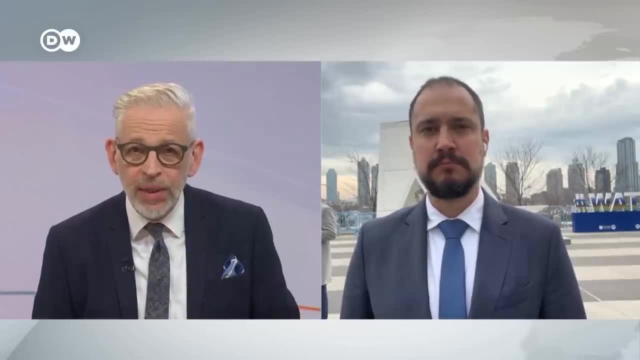 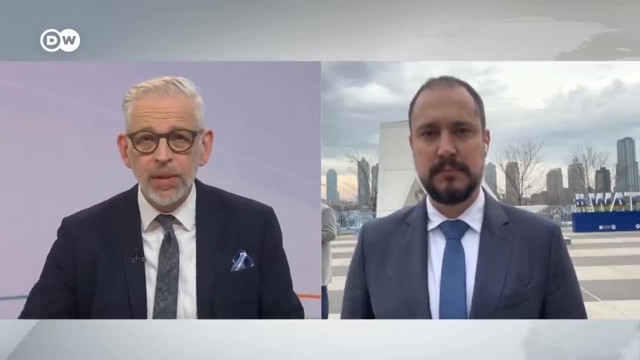 Sir, as the summit kicks off, the US government promised 49 billion US dollars of funding to help the global water cause. Will money really be enough to solve this issue? 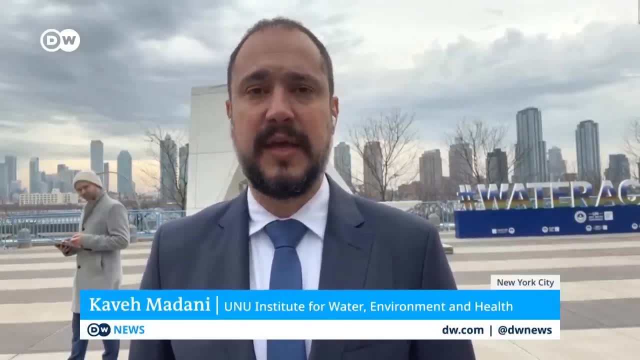 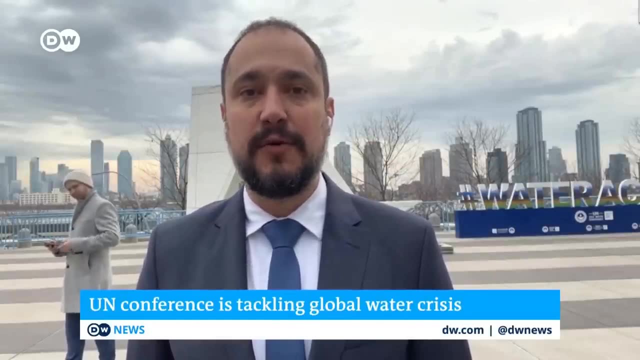 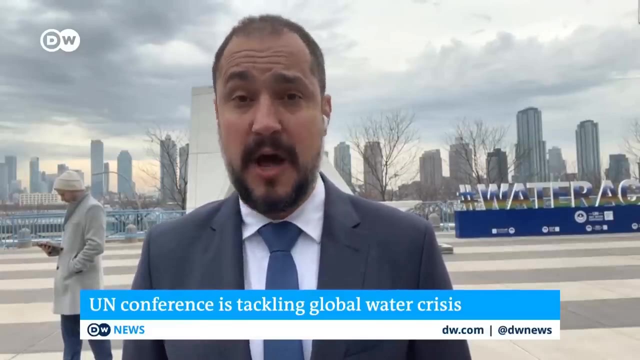 Actually, today there would be a report coming out that is suggesting that money is not going to solve the problem. Because besides money, there is a need for better planning, foresight, governance and understanding that this problem is a problem of common good. So one government alone cannot solve it on its own. 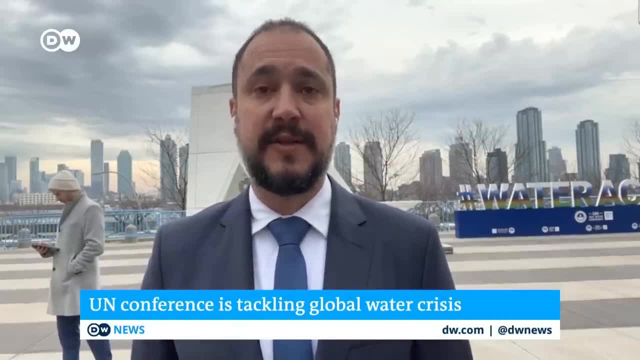 And whatever happens anywhere in the world can affect the rest of us living across this planet. 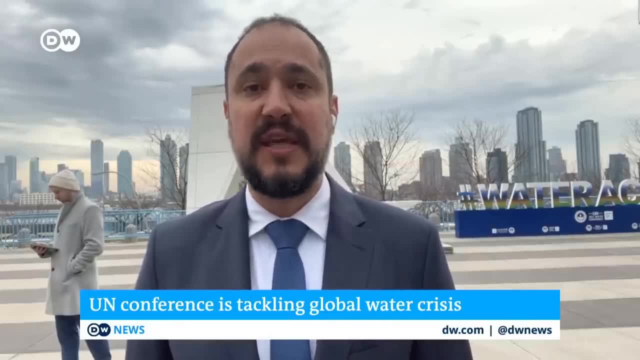 What we are hearing is that essentially three out of four people in the world 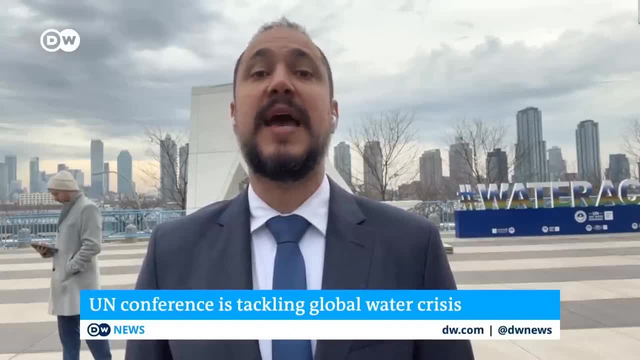 are currently living in the world. They are currently living in water insecure areas. 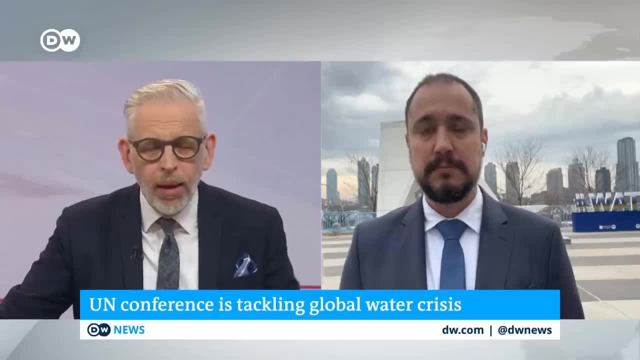 And this is quite alarming. When you say money is not the issue but planning is, what do you mean by that? 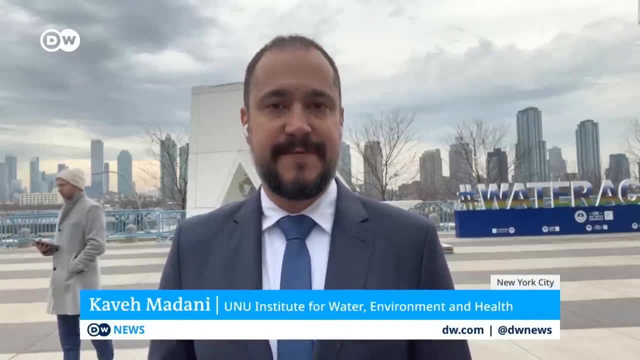 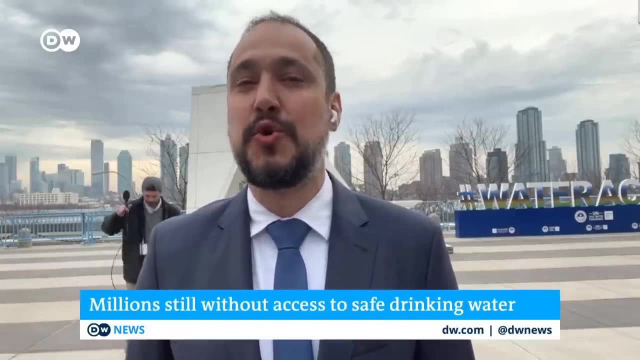 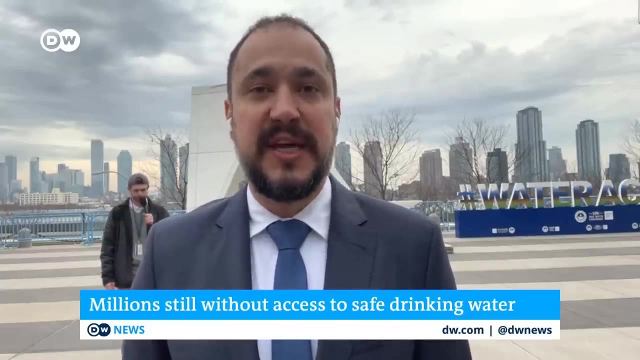 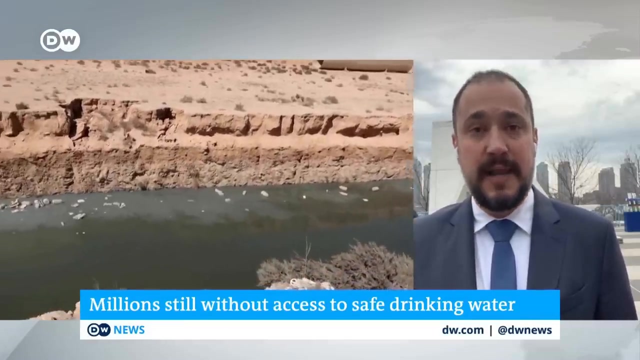 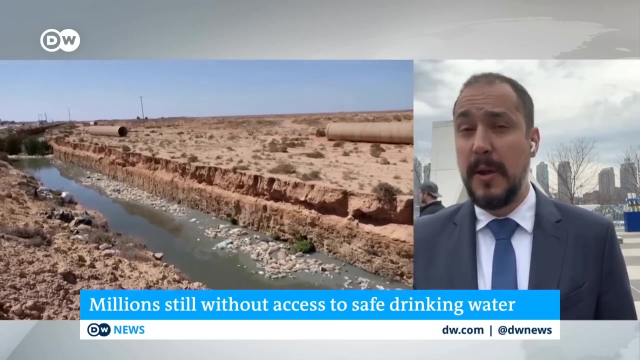 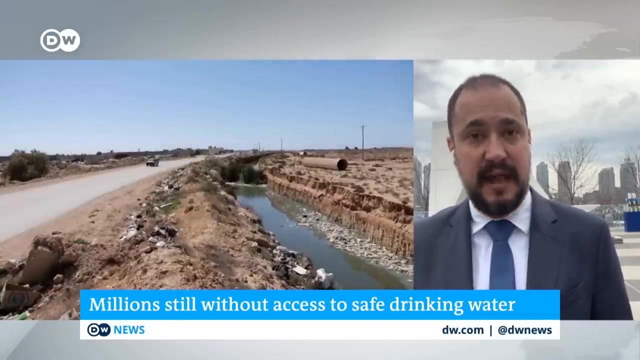 So I think we have seen it quite often that in rich countries, I mean rich regions of the world, still where there is no shortage of financial resources, and there are some homeowners who are using government-funded resources. But what we are hearing is that the strategy that people are planning is resulting in reservoirs that are empty, and growth in the water consumption and water demand and agriculture development. Farmers go and bankrupt food security being affected. And these problems are not the problems of the global South only, they are not the problems of Africa or South America or Southeast Asia. 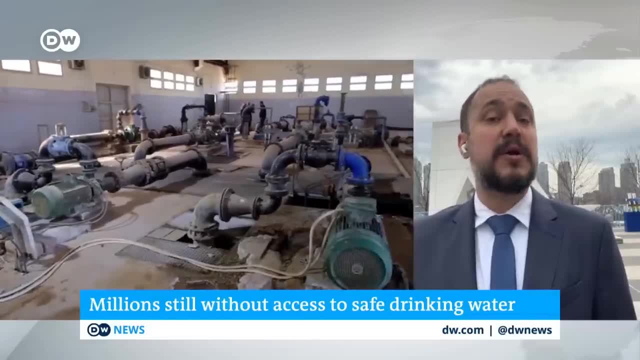 that I'm talking to you from. And all of this is because of the lack of force. We didn't certainly see water as a limit to growth, 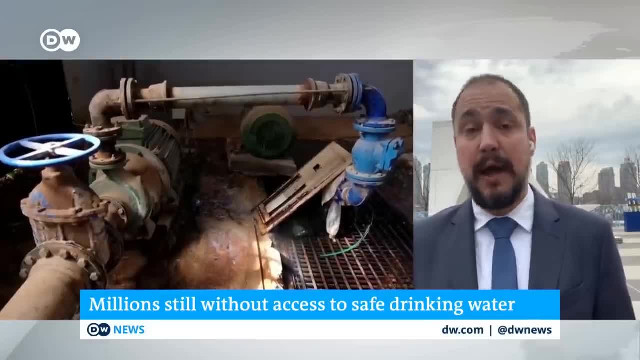 and we didn't plan for it properly. And now with climate change and all the changes that are happening, anthropogenic impacts of human development, the situation is getting worse and worse. 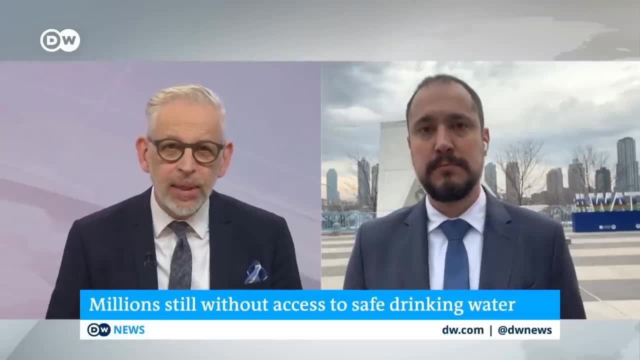 Now, just last year, one third of Pakistan was submerged in historic floods, leaving millions of people deprived of drinking water. 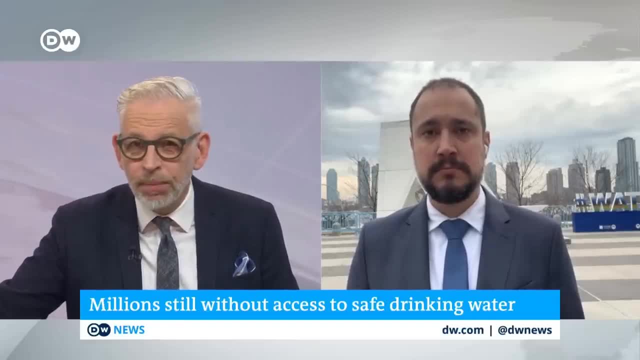 Do you expect events like these to happen more often? Absolutely. With climate change, we expect more extreme events. 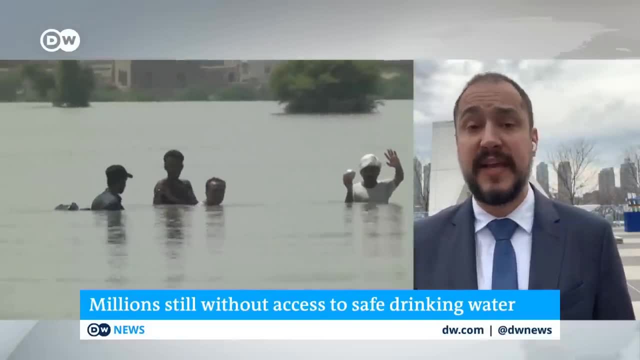 We have done the design and planning based on the historical data that are no longer valid. 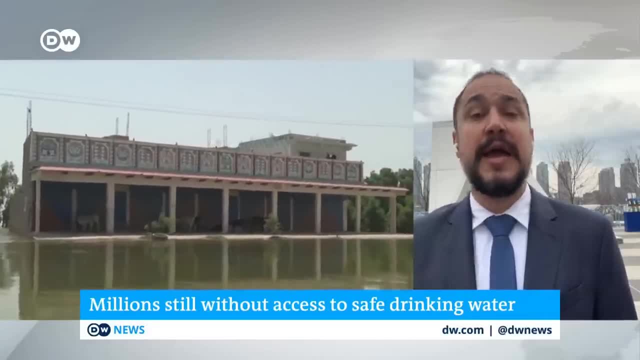 It's very hard for us to move people from one location to another. It happened in Pakistan, but let's not forget that in Germany, 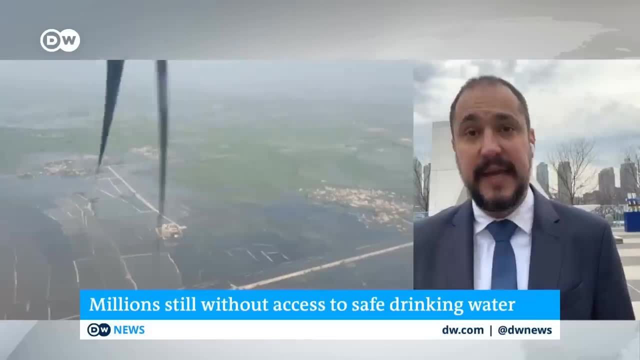 also we had a point that was quite costly. And this is the problem of both the global south and the global north. 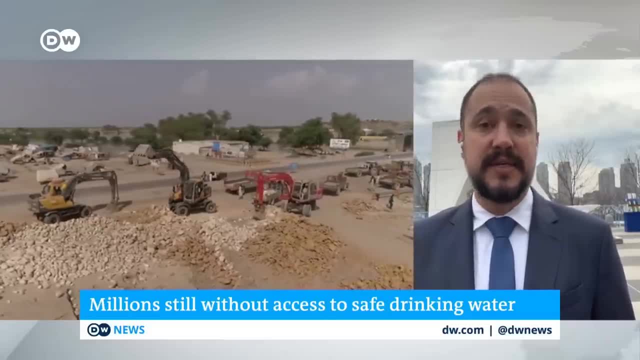 And in the future, I'm afraid the problem is going to get worse. It's still promising that after 46 years, 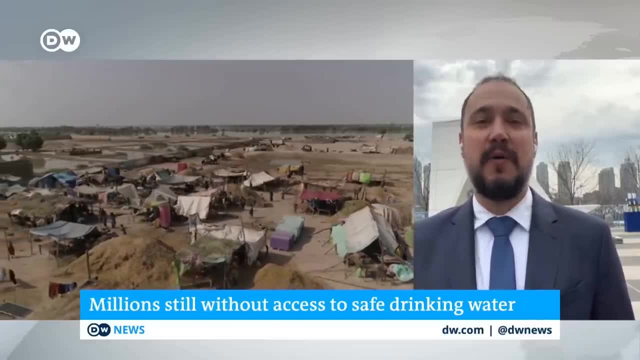 we're getting together here talking about water at another UN Water Conference. 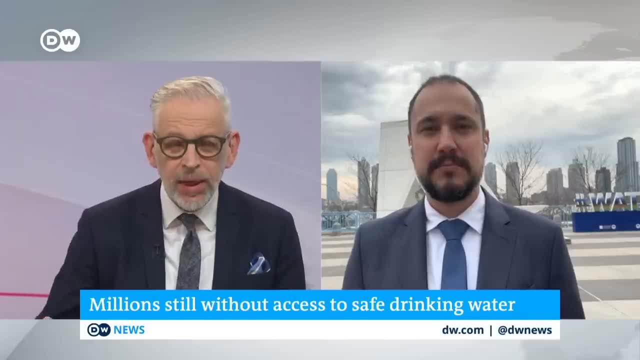 Now, you've been following the discussions there at the conference. Do you expect any real tangible outcome there? 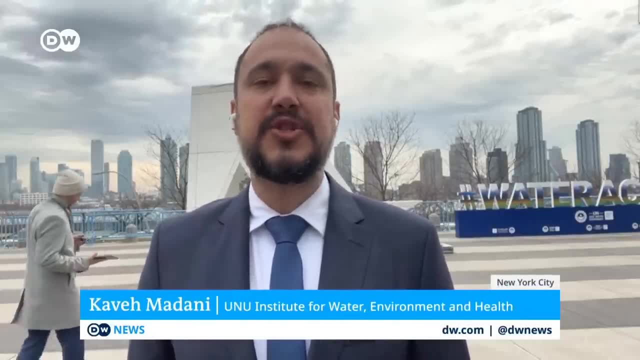 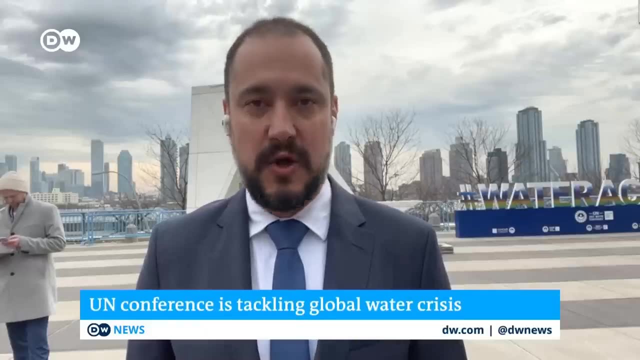 So that's a very good question. I think the Secretary General, is insisting on the fact that cheap talk is not going to solve the problems of this planet. 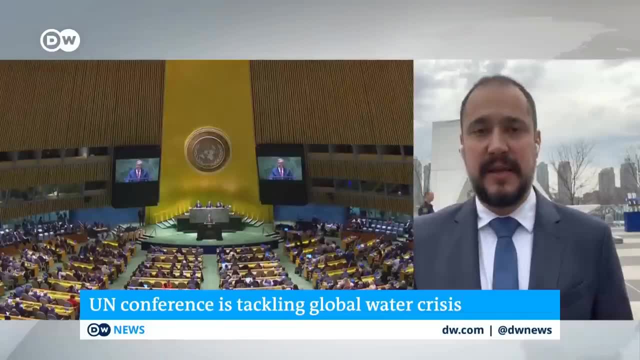 We have to do things differently. I think water in the next few years 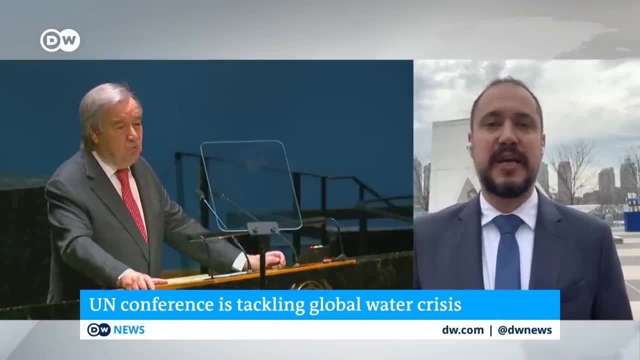 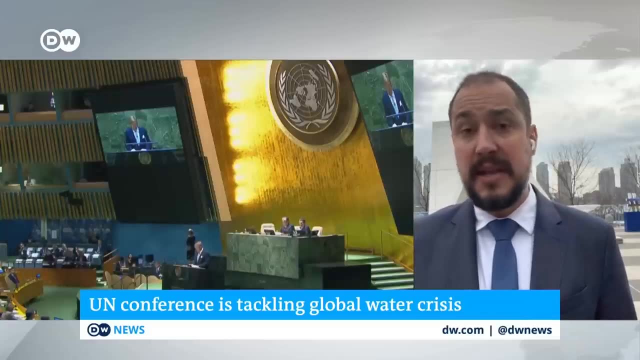 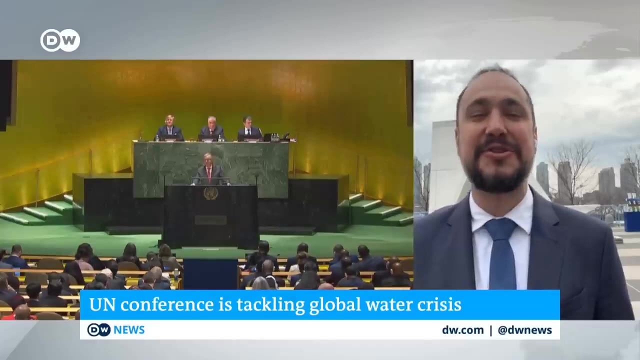 would be on the agenda of many UN agencies, including FAO, Concerned with Food, WHO, and many other agencies, because now we understand that whatever we want to do to fight climate change, to deal with biodiversity loss and to fight pollution, the triple planetary crisis, we have to make sure that we do something for water.